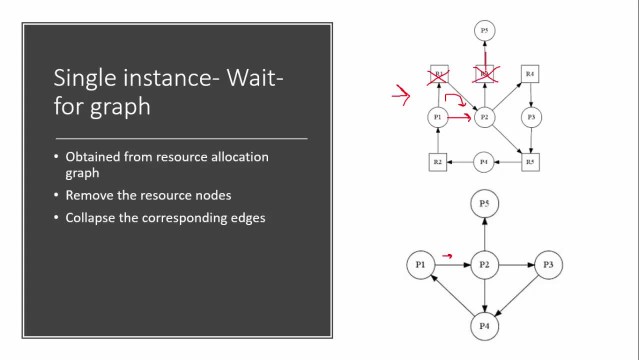 So we'll remove the resource and collapse this edge, So from P2 to P5.. Hence, to convert a resource allocation graph into a wait for graph, we are going to remove all the resource nodes and collapse the corresponding edges. Now, after doing this, if there is a cycle in the wait for graph, then the system is in a deadlock state. Otherwise it is deadlock free. 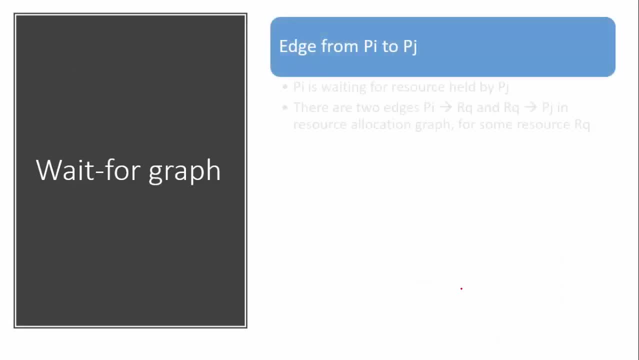 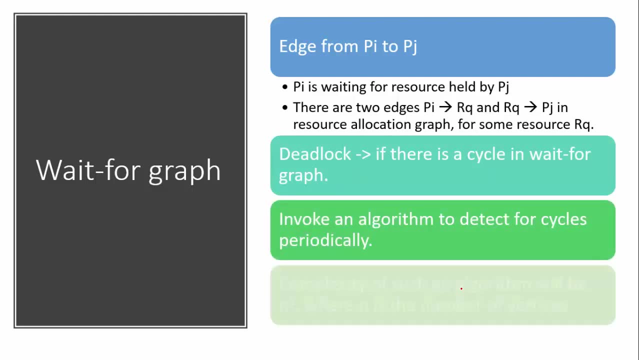 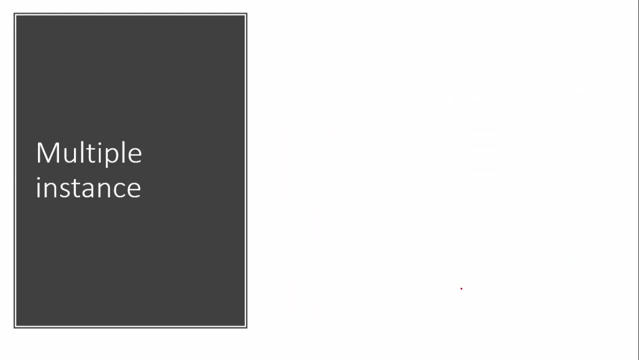 This is the end of this video, Thank you. This is the entire procedure that I have explained with the example. You can just pause the video and go through it once again Now. the wait for graph can work only if there is a single instance of each resource. 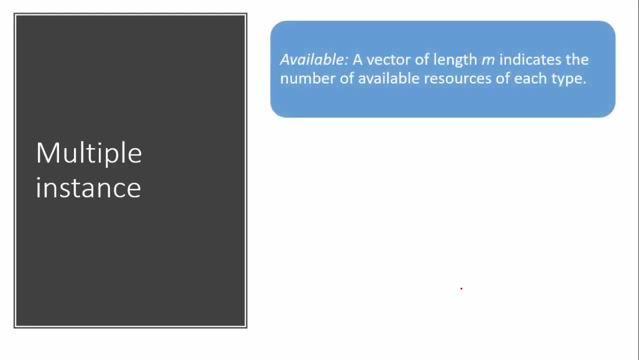 For multiple instances. we use a different algorithm which is similar to the Banker's algorithm. So if you have understood the Banker's algorithm, this is pretty straight forward. Here also, we are going to use a single instance. We are going to use three data structures available. 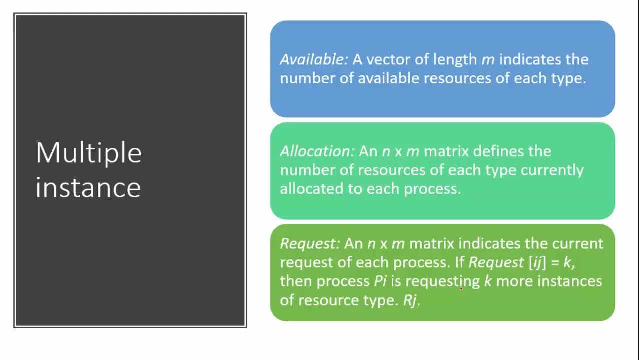 Available is the number of instances of each resource that are available with the system Allocation. This is the number of instances of each resource that are allocated to the process And request. Request is what a process can request in the future. So what resources can a process request in the future? 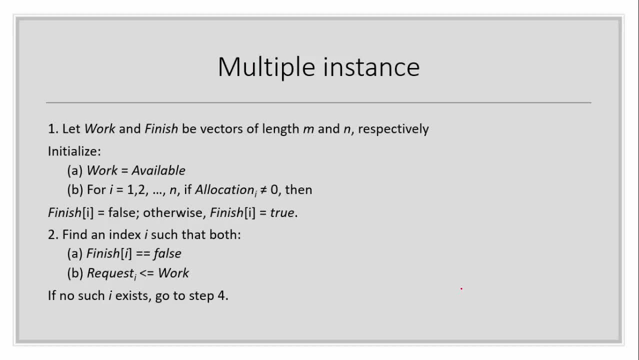 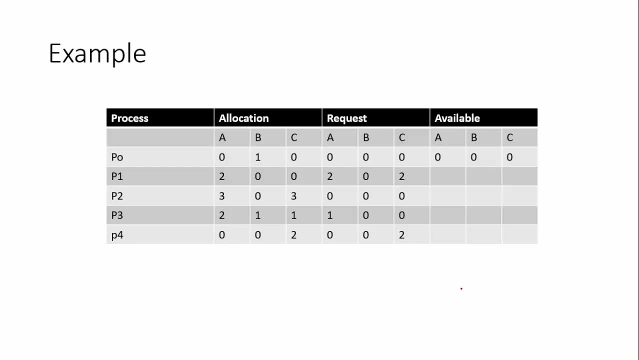 So this is the algorithm. I am going to explain it with the help of an example. So now there are five processes: The allocation is given, The request is given And the available is given. So the working is pretty similar to Banker's algorithm. 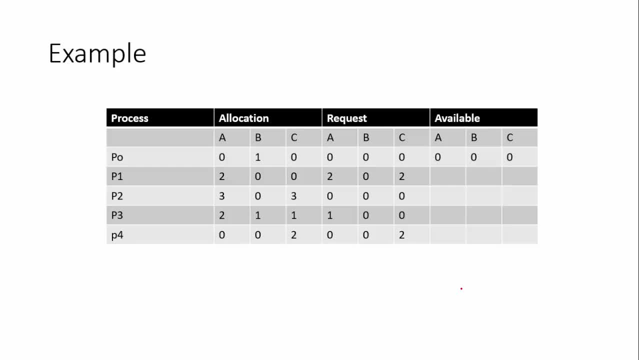 But now we are not required to calculate any need. The request is the need. Okay, What is the request It will request in the future Allocation? How many resources are there now? So P0 is currently holding 0 instances of A, 1 of B and 0 of C. 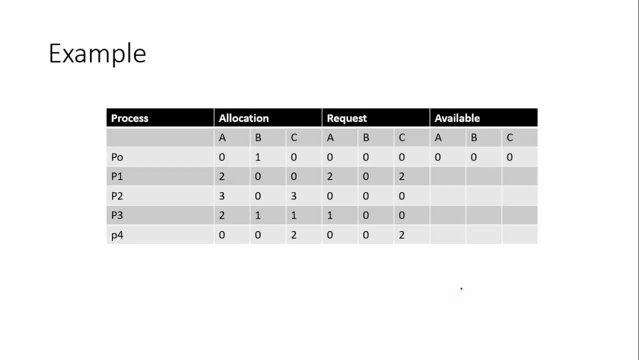 In future, it can request 000 of each. Similarly, for P1,, allocation is 200 and request is 202.. And for all other processes, The available number of instances with the system are 000 of each of the three resources. 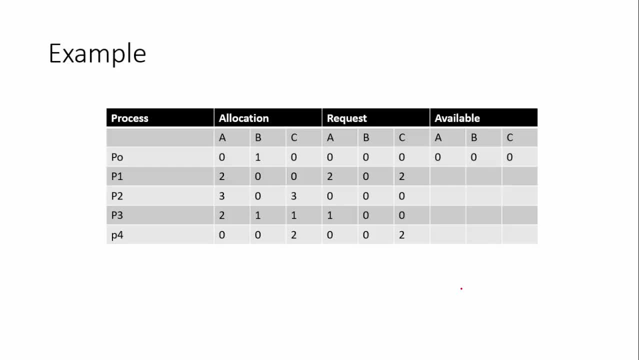 So now, what I am going to do is I need to come up with the save sequence. If we can come up with the save sequence, then the system is deadlock free. Otherwise, it is in a deadlock state. So now, if the system is in a deadlock state, let us find a process whose request is less. 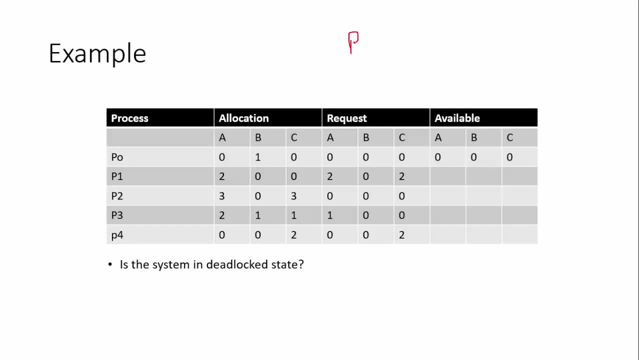 than or equal to available. What I am going to do? I am going to find a process whose request is less than or equal to the available. So P0 is one such process. Request is equal to available. Now, once the request is satisfied, this means that I am going to update the available by 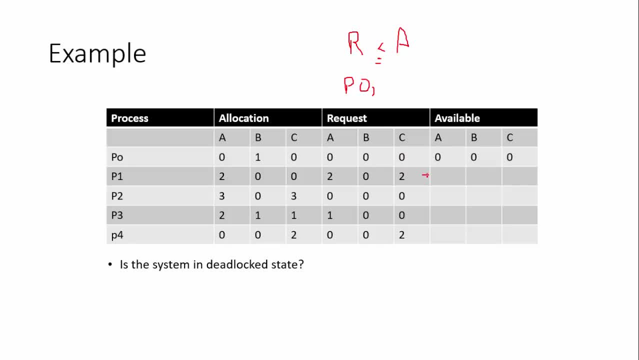 adding the allocation. So we can allocate, we can update the available by adding the allocation. So now the new available is 010.. Now find out another process whose request is less than the new available, which is 010.. So the new process is: is it P1?? 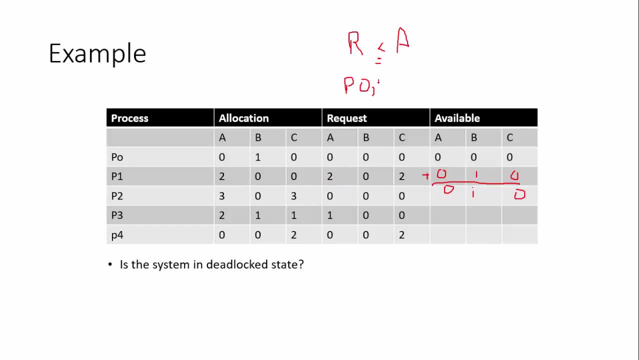 No, Is it P2?? Yes, The next process is P2.. Once P2 is finished, we will update the available by adding the allocation of P2, which is 3,, 0 and 3.. So the new available will be 3,, 1 and 3.. 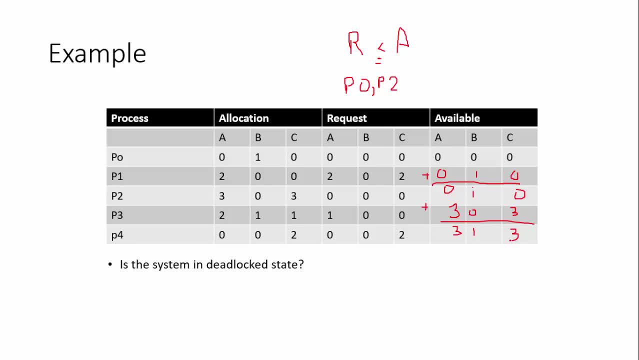 Now find out the next process, So P3,. can we satisfy the request 100?? Yes, So the next process is P3.. So, in the same manner, we are going to move forward and we will see that we are able to. 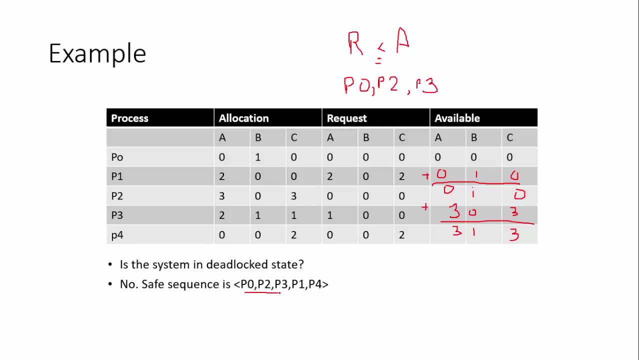 come up with the safe sequence, which is P0, P2, P3,, P1 and P4.. Since we are able to come up with the safe sequence, this means that the system is not in a deadlock state. Now the next part will be P2. request one additional instance of C. What we are going to do is: 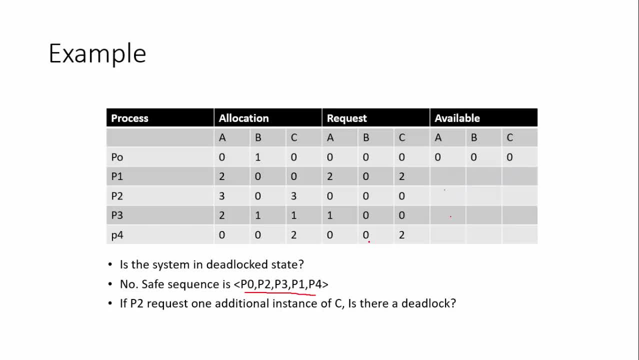 it is requesting one more instance of C. So what is the current request? So what is the current request of P2?? It is 0, 0, 0.. Now, according to the question, the new request is what One additional instance? 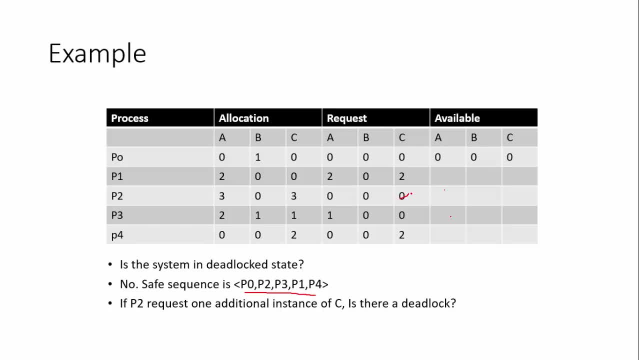 So it is going to be 0, 0 and 1.. So this is the scenario. Now let us try to come up with the safe sequence once again. So P0 is the first process whose request can be satisfied. So P0 is our first process in the sequence. 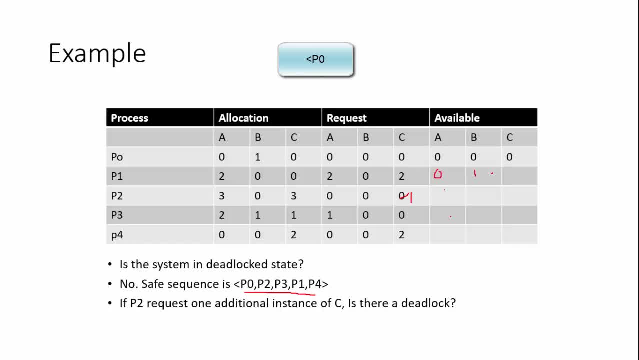 Update the available by adding 0, 1.. 0, 1 and 0. So the new update available will be 0, 1, 0.. Now is there a process whose request is less than or equal to available? 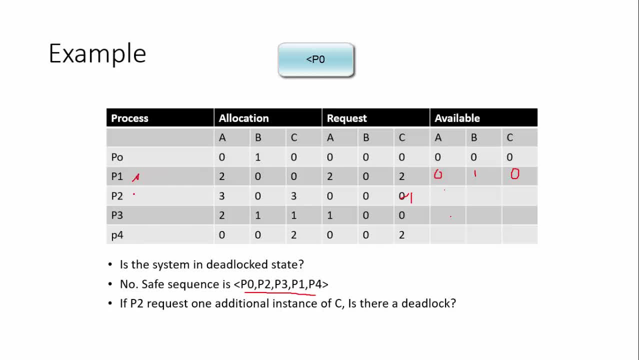 Can it be P1? No, Can it be P2? 0, 0, 1.. We do not have 1 for C. This means we cannot satisfy P2.. P3? 1, 0, 0.. 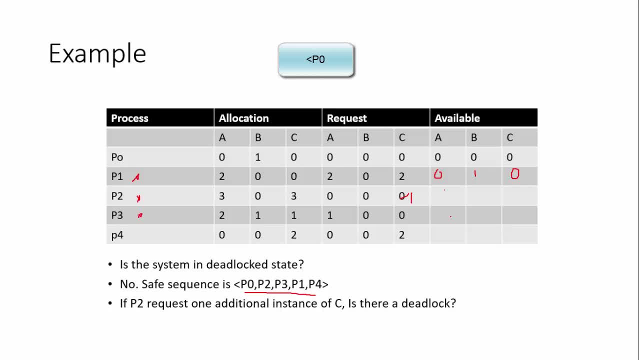 We do not have one instance of A- Again no. P4 is 0, 0, 2.. Again no. This means that we are not able to come up with a safe sequence if P2 requests one additional instance of C. Hence the system is in a deadlock state. 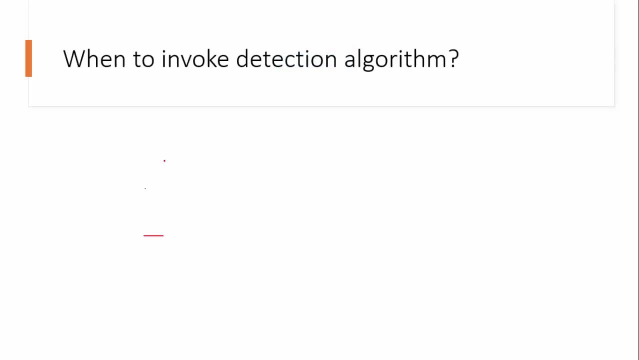 Now the next question is when to invoke the detection algorithm. When do we invoke the detection algorithm? There are two possible ways. First one is you invoke every time a process requests for a resource. Then we will call the detection algorithm. Second method is you invoke the algorithm after a fixed interval of time. 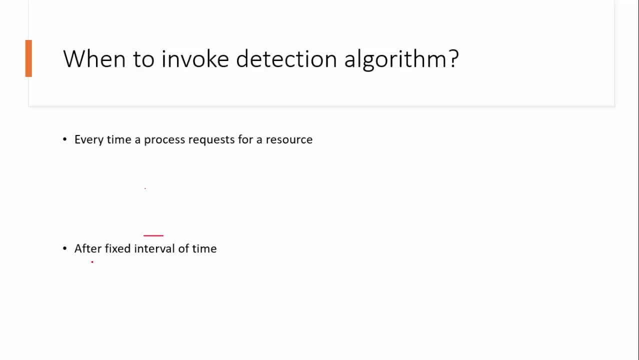 After every half an hour or after every one hour, It depends. So you invoke it after every fixed interval of time. Now let us see what is the advantage of the first technique Every time a process requests for a resource. So what can be the possible advantages? 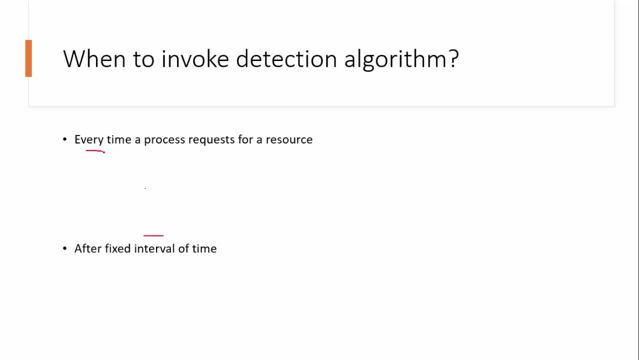 The first advantage is you will be able to identify that which processes are involved in the deadlock. Right The JSI request query, the algorithm is invoked and you detect. okay, fine, The deadlock has occurred due to this particular request and these processes are involved in. 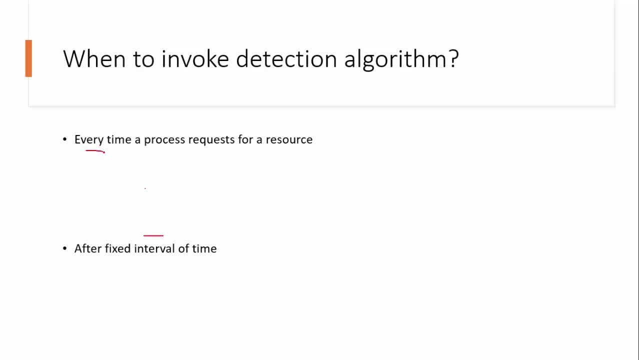 it, So you are able to detect which process has caused the deadlock and which processes are involved in the deadlock And what is the drawback, Since you are going to call it every now and then. there are lot of processes running in the system And they are continuously requesting for resources. 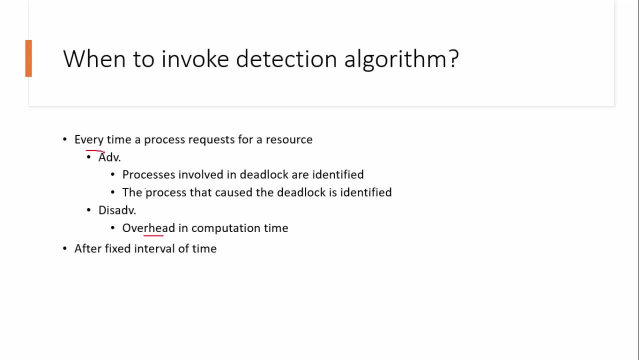 So invoking the algorithm time and again will be a overhead in the computational time, Because the longer you are detecting it, the longer the system will use it. So there is no useful work happening in the system. So that is an overhead. Now coming to the second method, 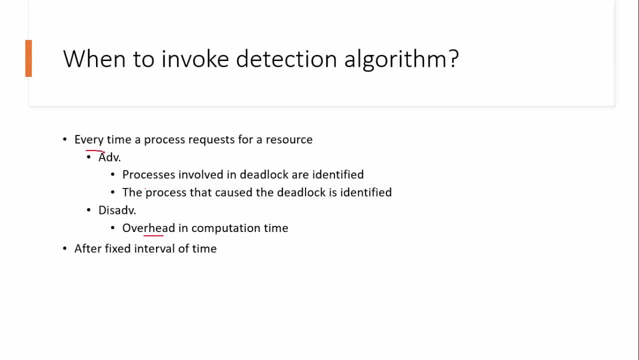 Invoking it after a fixed interval of time. So what will be the advantage? The advantage is that the overhead will be reduced. You are going to invoke the algorithm after, let us suppose, once in one hour. So you will invoke it once in one hour and it will not waste much time. 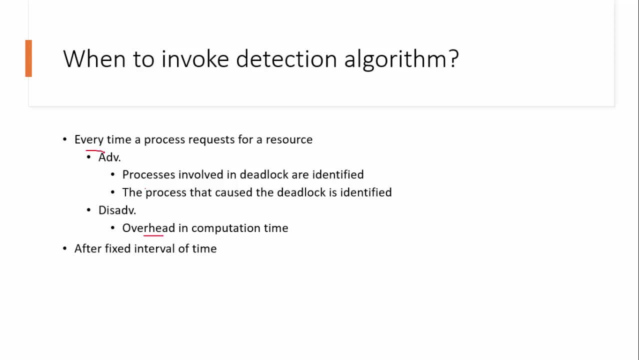 So that is the advantage part And what is the disadvantage? Obviously, you will not be able to tell that which process has caused the deadlock, Because let us suppose it is 10 o'clock and you have invoked the algorithm At that time. there was no deadlock in the state. 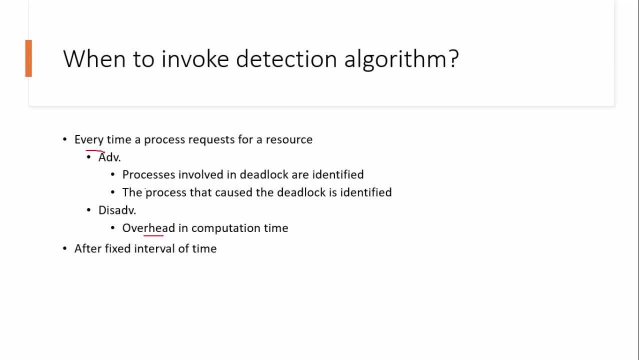 At 10.05 the system enters into deadlock, But now you are going to invoke the algorithm at 11 o'clock, So you will not get to know till 55 minutes, And during that 55 minutes a lot of other processes might take place. 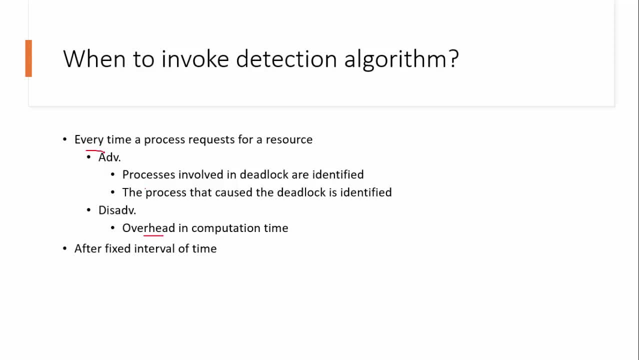 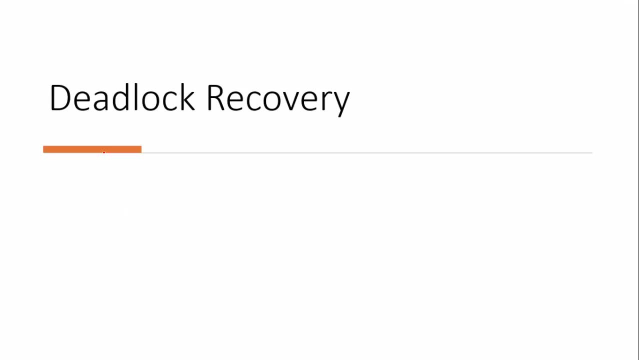 And hence you will not be able to tell which process has caused the deadlock. Last part: Once you are able to detect the deadlock, This means now you need to recover from it. If the deadlock has been detected, Now what you have to do? 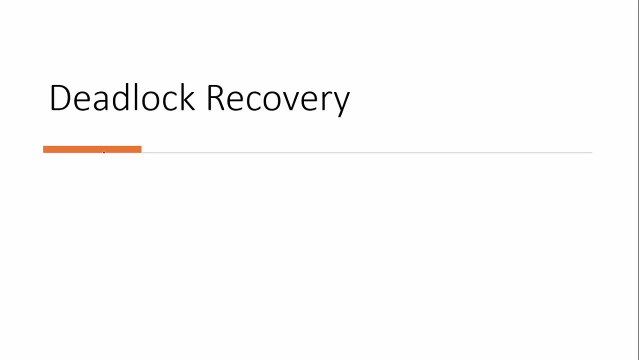 Come out of the deadlock. So what is the method that you invoke? You must have faced the deadlock many times in the system. Deadlock is what. Whenever your system gets hanged, That is the situation of a deadlock. We have seen this many times in our laptops and phones. 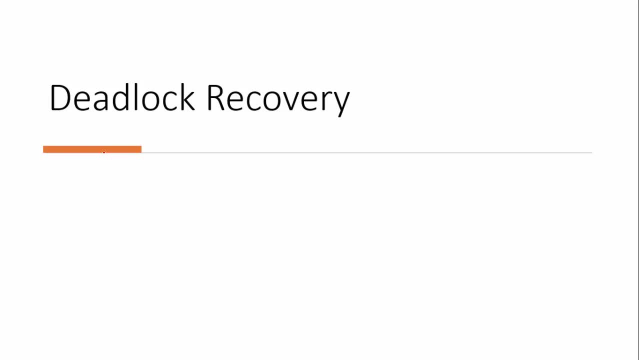 So what is the best method? that we do, Yes, We restart the system Right. Or sometimes, what we do, We do control all, delete. We open the task manager And then we kill a few processes that are not responding. We kill the processes that are not responding. 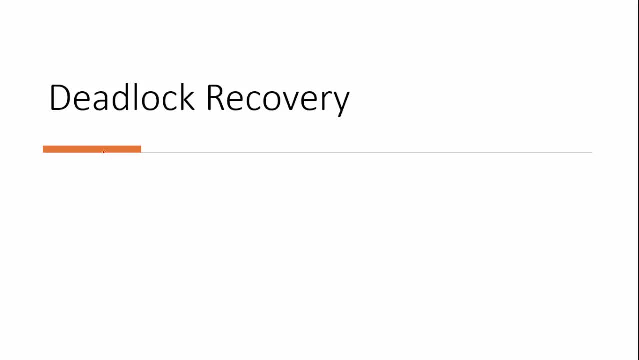 Okay, There are two techniques to recover from deadlock. One is process termination And second is you preempt the resources from some of the deadlocks process. Either you kill the process Or you take back some resources from the processes. Now what are the challenges in each of these techniques? 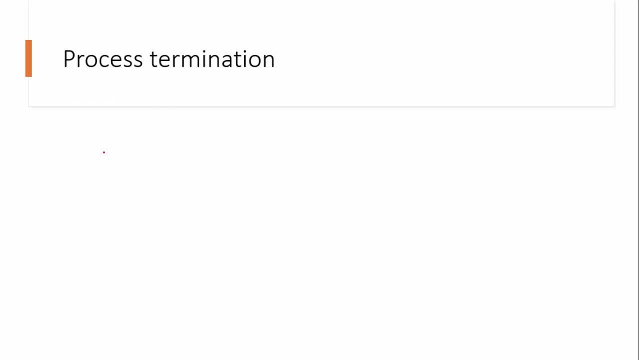 Process termination. So in process termination there can be two methods. One, You terminate all the processes, All the processes that are involved in the deadlock. You terminate all of them. So obviously automatically the deadlock will be broken. Second is You kill only or you terminate only a few of them. 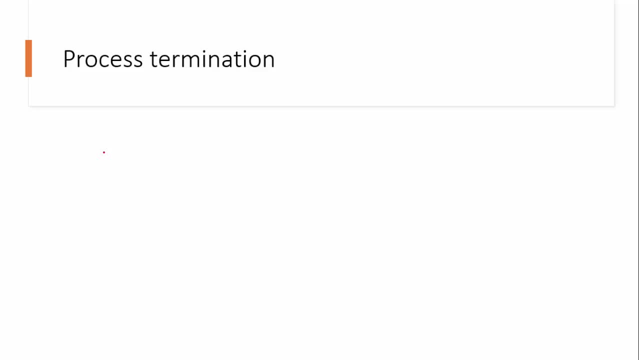 Kill one, See if the deadlock is broken. If not, then kill two, And so on. Now the question will come: Which one to terminate? Okay, Now that is a. There is no fixed answer to that: Which one to kill. 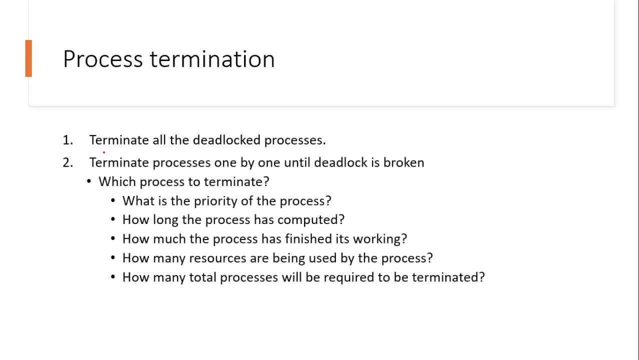 There can be different reasons, Depending upon the state of the system or the processes that are running. For example, At this time you want a process which is almost 99% completed. You don't want to kill it, Right, But sometimes you might not want to kill a process which is of highest priority. 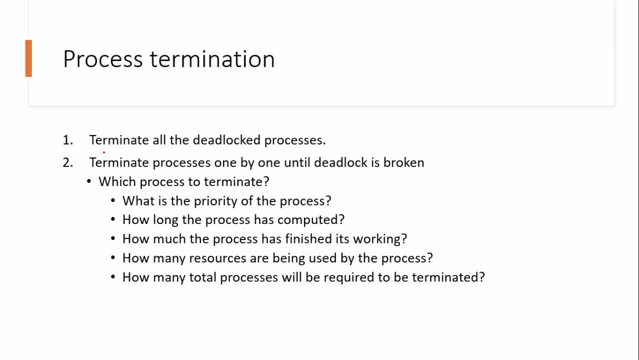 Even though it has run only for, let us suppose, 10% of its total execution time, So it has a higher priority. Maybe you don't want to kill it, Right? So there can be different reasons. A few of them are mentioned here. 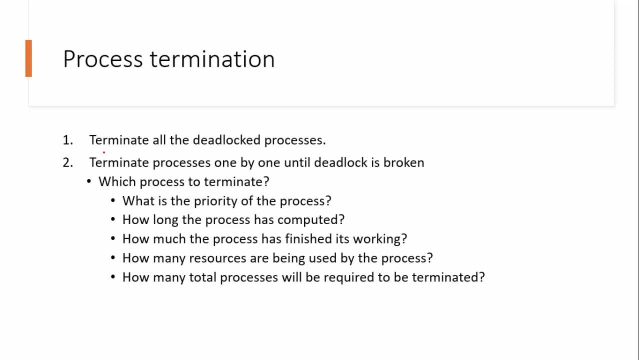 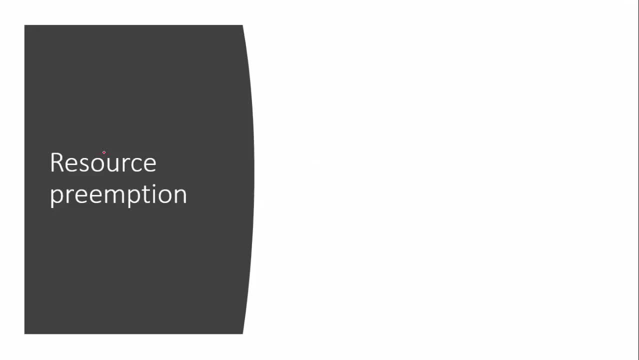 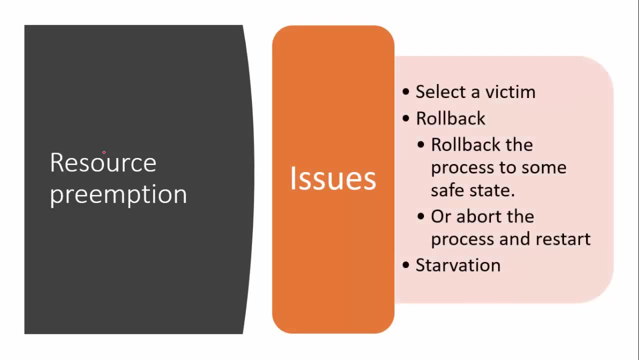 So there is no fixed answer to that, Which one to kill, That is up to you. Second technique was Resource preemption. Now, in resource preemption again, there are certain issues. First one is: Select a victim Again. From which process do I return the resources? 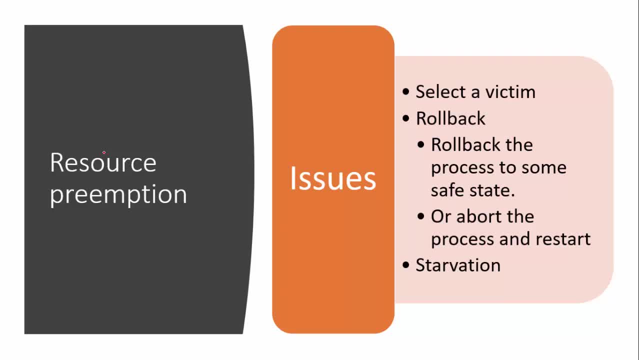 So the reasons can be different as in process termination. Second is Rollback. If I am going to take back resources from the process, This means that the process cannot continue with its normal execution. So it cannot execute normally. So maybe that process will be in the middle of the transaction. 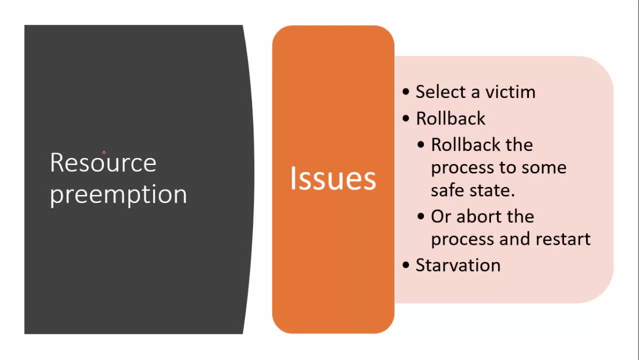 This means I need to take it back to a safe state Right? So during the rollback, Either you take back the process to a safe state Or You abort the process and then restart it again. Third thing is Starvation. You must ensure that the same process is not always selected for resource preemption. 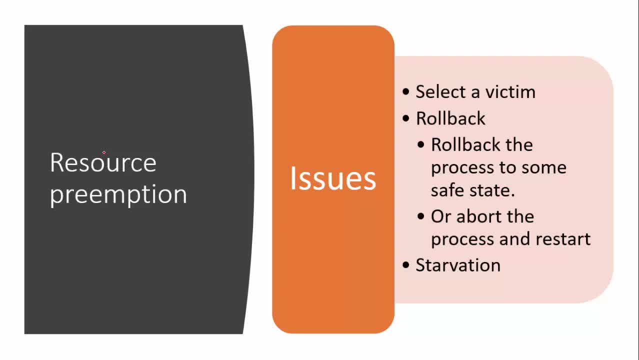 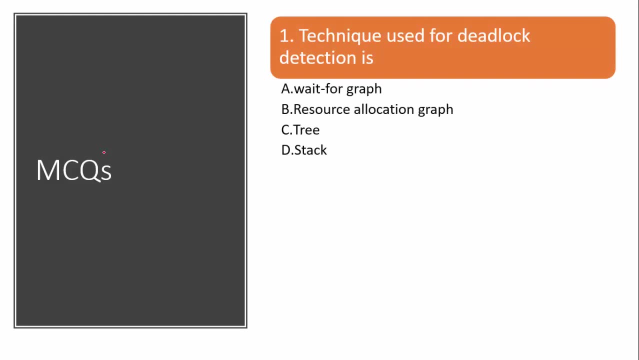 Every time when there is a deadlock. Do not preempt resources from the same process again and again. This must be ensured. So these are the three issues in resource preemption. There are a few MCQs For you to practice, Apart from MCQs. 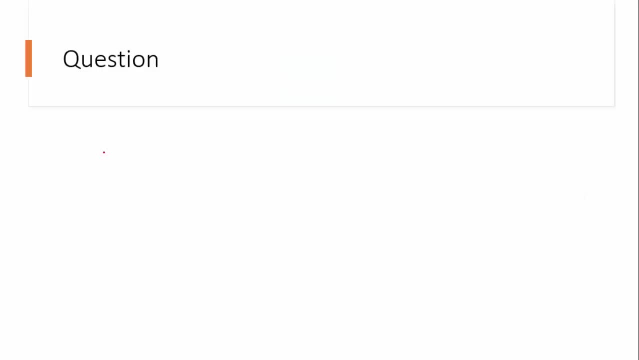 I have seen a very common question that is asked generally in UGC net or GATE exam, So I am going to discuss that question. The question is: A computer system has six tape drives And N processes Competing for them. Each process may need three tape drives. 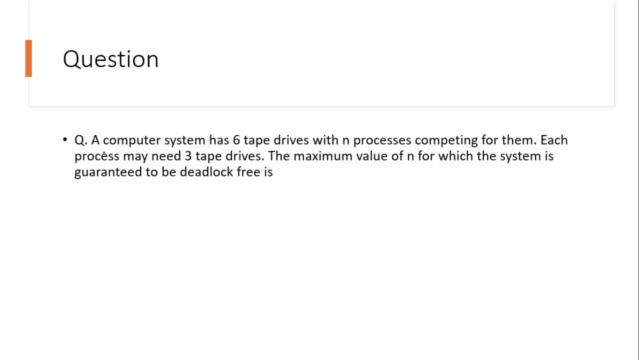 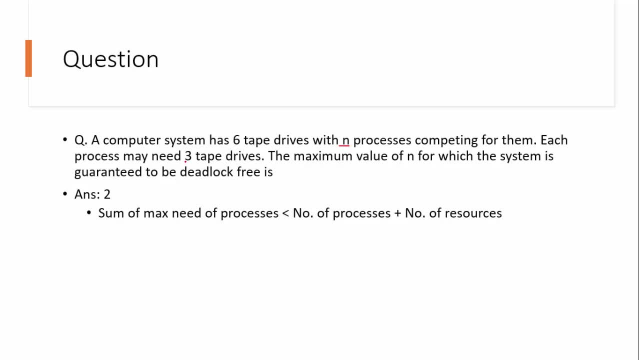 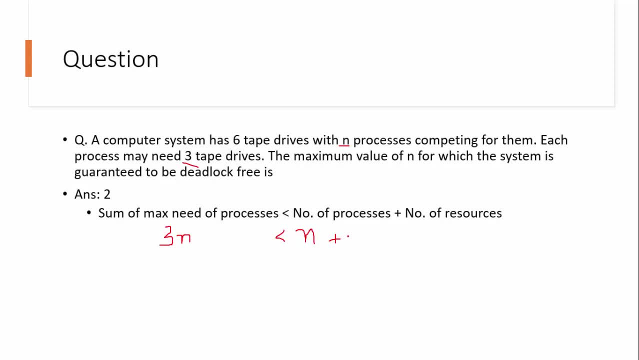 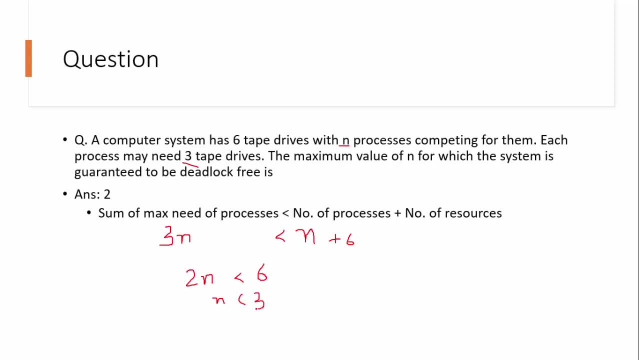 3. so what is the value of n less than 3? maximum value is 2, hence 2 is my answer. okay, so remember this formula: sum of max need of processes should be less than number of processes plus number of resources. so i hope you have enjoyed these videos on deadlock and its related.